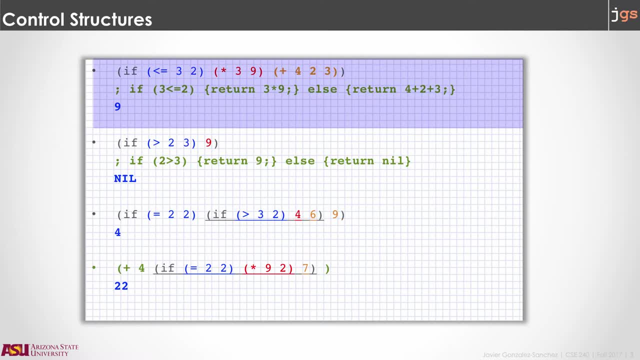 happen is that the result of the function that is being executed- multiplication or addition in this case- is going to be returned as the value of the full line. So if you run this line, what you are going to have as a result is the number nine, and the reason is because the condition is false. then the 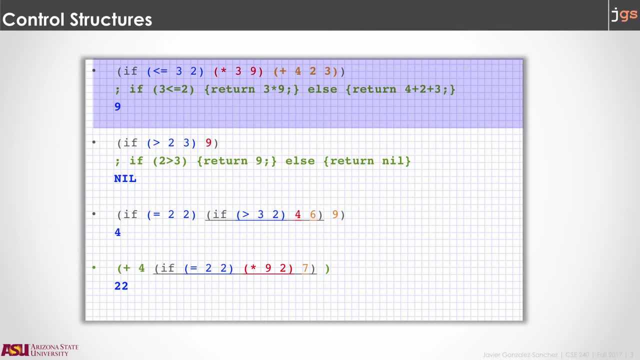 function that have the plus symbol at the beginning is going to be executed, and that is four plus two plus three and that is going to be the nine. The second example, again the name, if this example have only two parameters, so you can think about this as an if condition without an else. 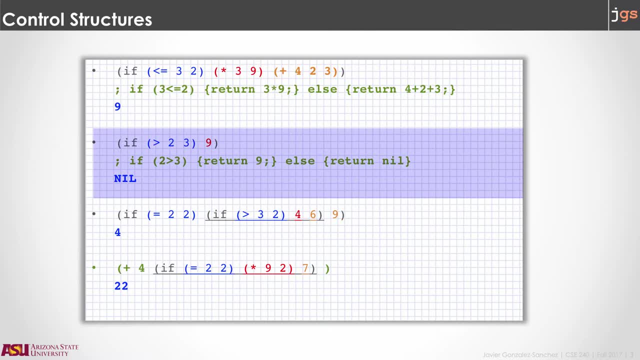 or with the else empty. So in this case, the condition is going to be reviewed if two is greater than three. If the condition is true, the statement is going to print nine. however, because the condition is false, the result is going to be nothing and that is represented as nil. Also, you can use another if 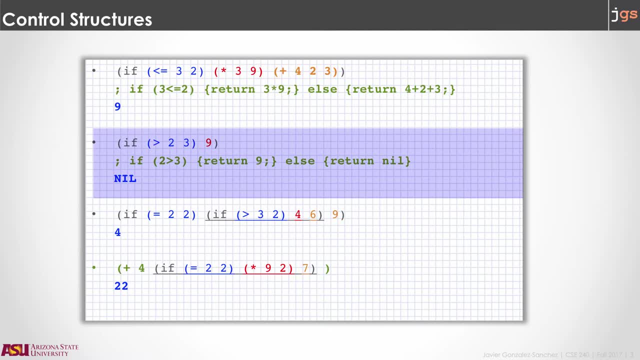 instruction as one of the parameters for the first one. so in this example we have an if structure. the condition is a completion between two and two, so something like if two equals two and, as you can notice, the first option after the condition. the parentheses got inside. 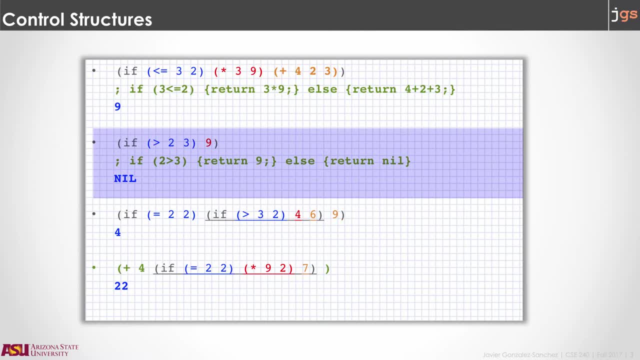 another if condition, Because the condition is the next element. it is into this line and in this level. the last oneити the condition is true. you are going to execute the list after the condition. so you are going to execute if and the new condition, 3 greater than 2, because that. 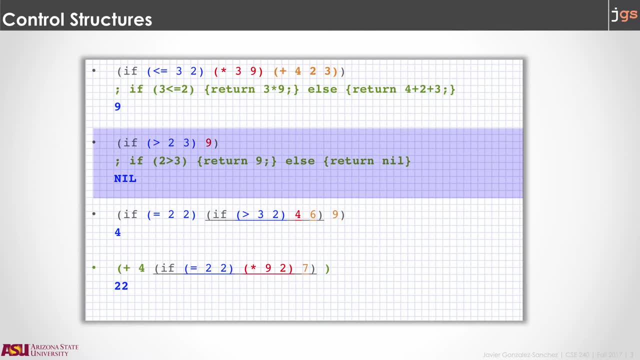 is true. you are going to return 4 and that is going to be the result of the line. Finally, because the if return as a result, then you can use the if as a parameter. for instance, here the addition is 4, the result of the if. so in order to do the addition, we need to calculate the. 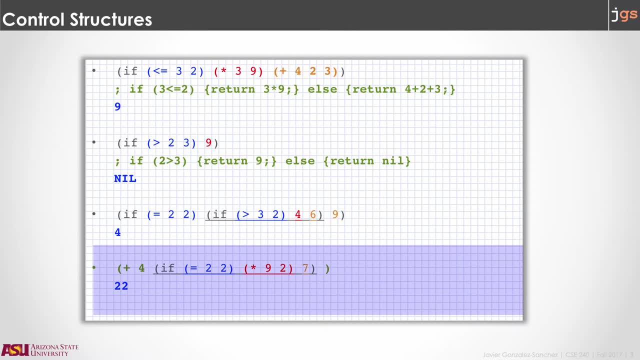 result of the if. The result of the if is going to be: first check the condition: 2 equal 2. that is true. therefore, you are going to do the multiplication of 9 times 2. that is going to be 18. that is the result of the if 18. and then you add 4 and the full. 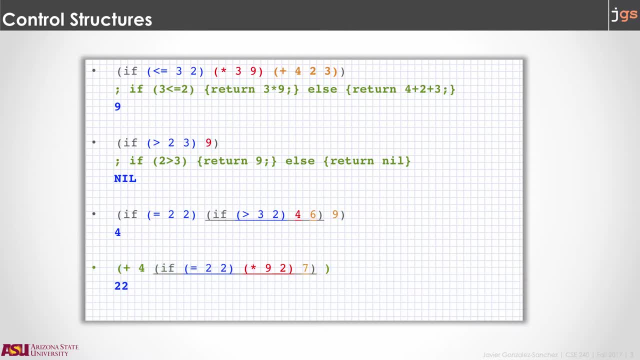 result of that line is 22. as you can notice, in all these examples the if and the else section are used- one line. that mean if the condition is true, you execute one line and only one. if the condition is false, you execute one line and only one. so something that we could need is the ability to put together 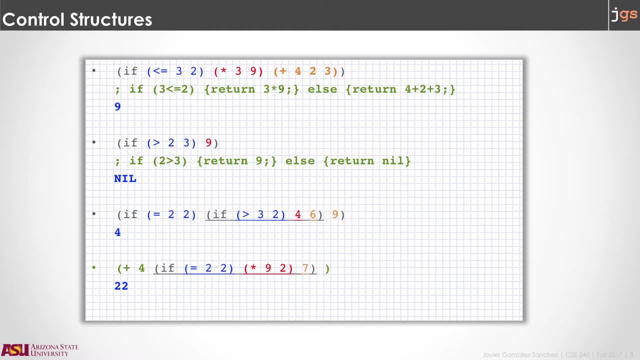 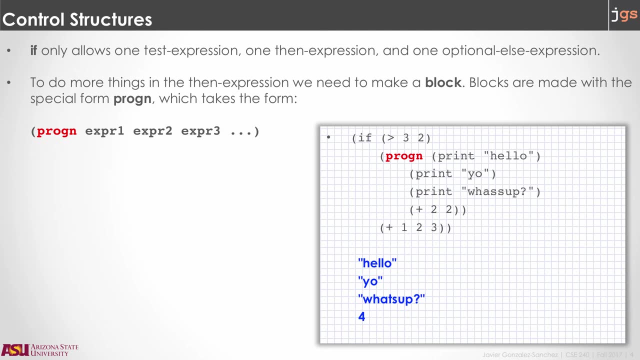 several lines to create a block and then use that block for the if or for the else. we can create a block using a list. with the keyword progn. you create a list, the progn is the first element in the list, and then each of the following parameters can be a list, and each of 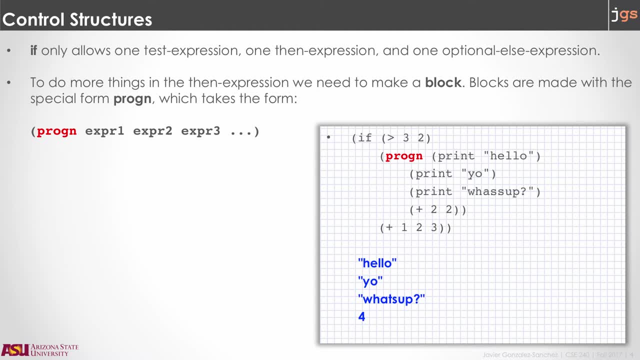 them could represent one instruction, then you can use all that as one parameter. for instance, here we have this if condition. the first parameter for the if condition is the condition itself: 3 greater than 2. the next parameter is this block progn that have four instructions inside and then the addition of 1, 2 and 3. 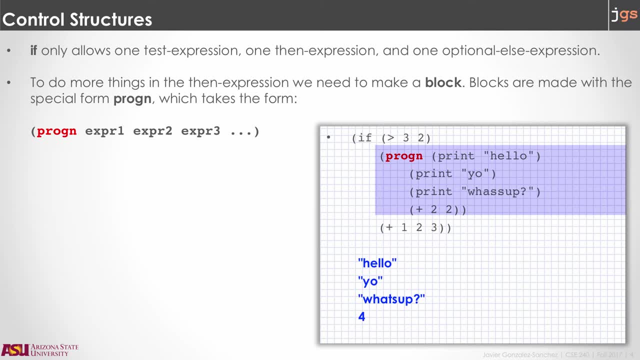 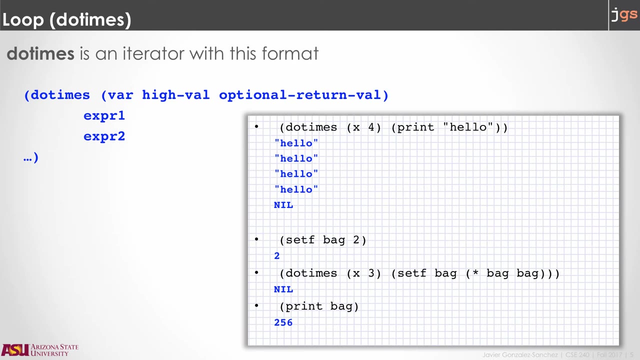 is the third parameter inside the list that begin with the if keyword, so that condition is equivalent to this block in C or C++. to create a loop statement, we use a list that begin with the keyword do times? do times have an infinite number of parameters, but the second parameter is a. 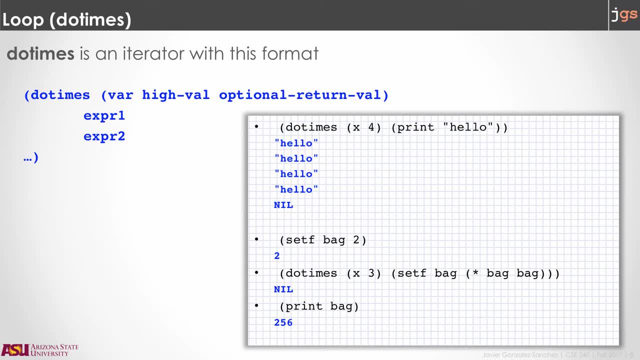 list, and inside of that list, we have three elements. the first one is a variable, the one that we're going to use to count. the second one is the higher value for the variable. and the next one is optional and is a return value. if we do not use this parameter, the default value as 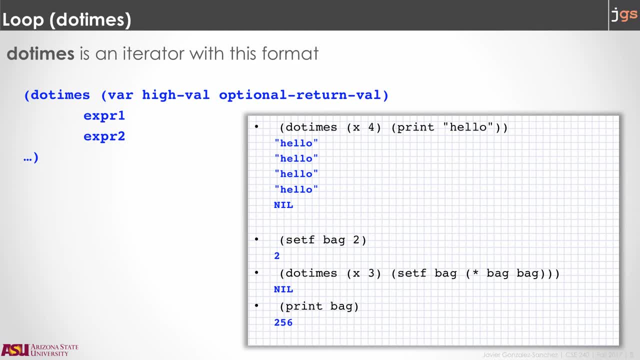 before is going to be nil, so the return value for the doTime list is going to be nil. the return value for the list is going to be nil, so the return value for the doTime list is going to be nil. after the second parameter, all the others are going to be instructions. 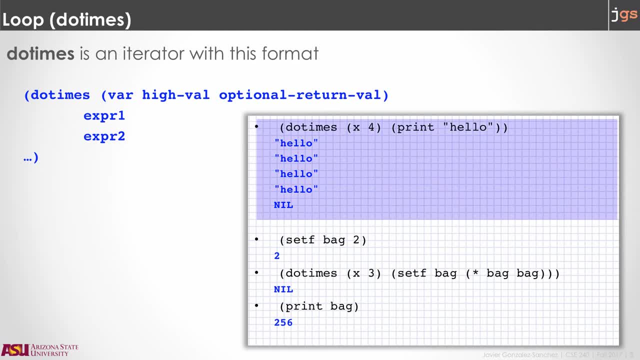 inside the loop. so, for instance, this example: here is a loop: we use a variable X as a counter and we are asking the loop to execute four times. so four is the highest value that we want for the variable and the loop have inside only one instruction, and that instruction is to print hello. therefore, when you run, 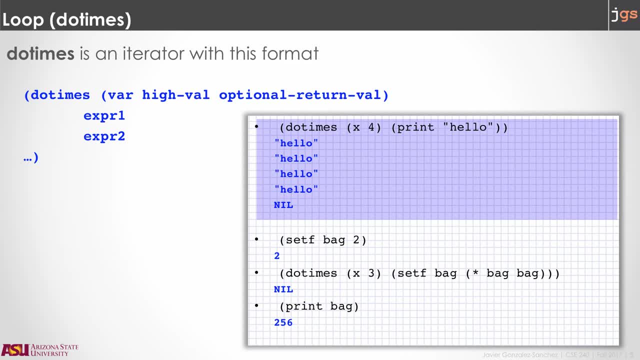 this statement, you're gonna have four hellos on the screen and at the end the nil represent the value that is returned by the statement do times. so you have the prints with hello and you have the return value of the times. that is nil, because we only specify X. 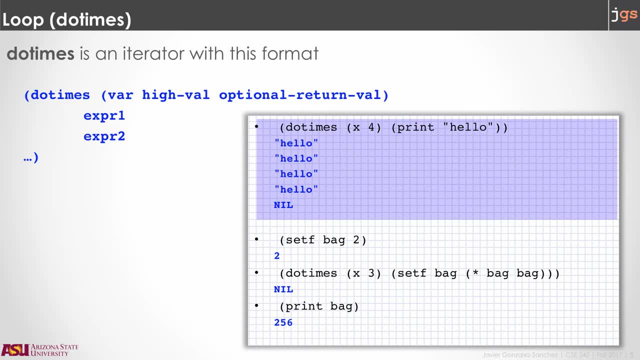 and for- and we do not put after the for the optional return value. so an equivalent source code in C could be something like this: and this could be the equivalent source code for the second example. in this second example we are creating a variable, a global variable we're going to talk more about. 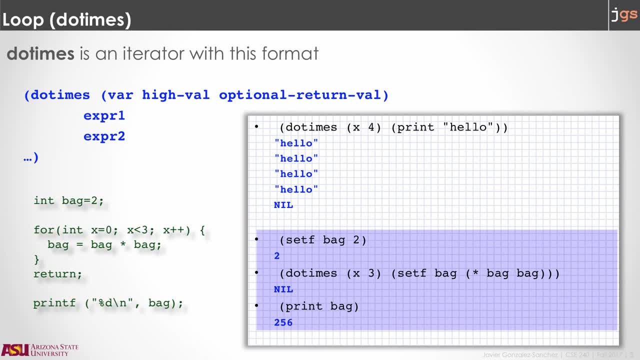 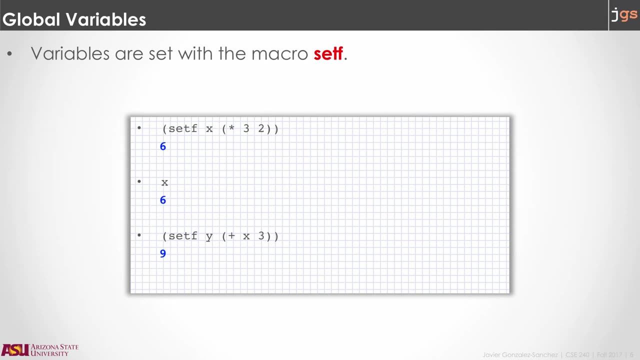 that in the next slide. but here, basically, we're using the variable to calculate something inside of the loop and finally we print the value of the variable on the screen. using ZF, we can define a memory location. ZF. allow us to assign a name to that. 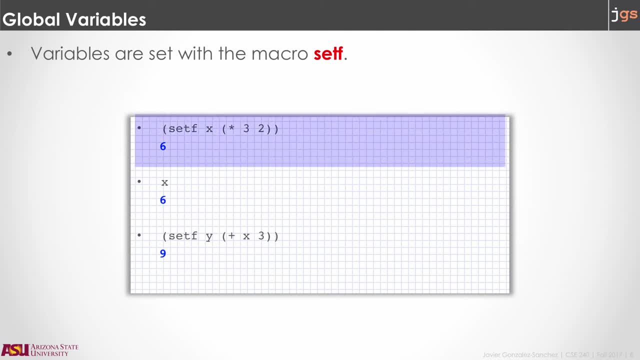 location and a value. so in this first example we are defining a location X and we are storing the value six in that space, because that is the result of the multiplication three times two. in the second example we are defining a location Y and storing the value nine there, because that is the 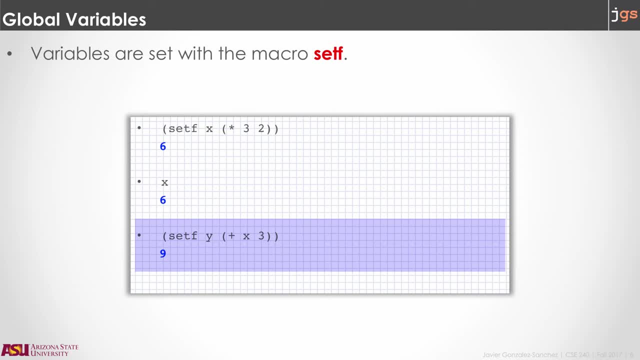 result of the addition between six, that is the value in the location, X plus three. when you define a name for a location, you can use that name as a value. also, if you type that name in one line of the interpreter, the interpreter is going to show you the value stored in that location. so typing X and pressing enter. 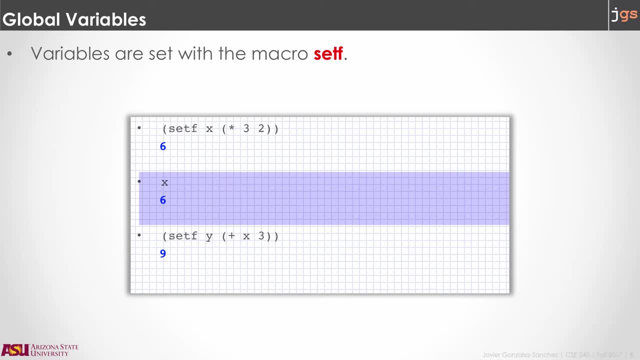 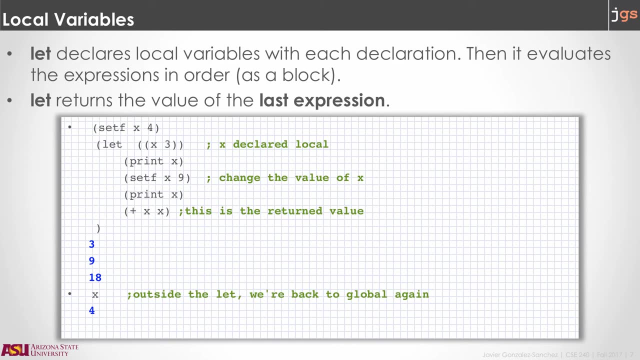 will print the six also that is possible to create something equivalent to local variables using the keyword let at the beginning of a list in the let list. the second argument is a list with lists with the names and value for the variables that we want, because what is expected is a. 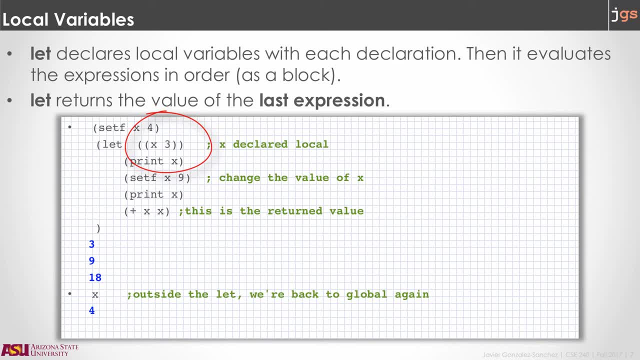 list. with lists, even though you only create one variable, you need to provide the open and closing parentheses for the list and the open and closing parentheses for the element after that list of symbols and values, kind of local variables. the other elements in the let list are instructions and those. 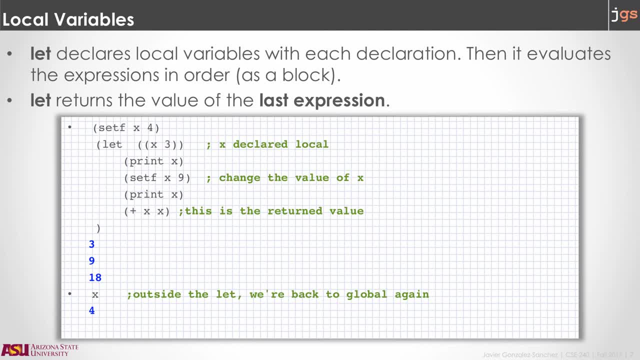 instructions are going to be able to use the symbol that we define as a local value. So in this example we can print x and that is going to print 3. We can use x in an assignment using setf and that is going to put 9 as a value in x, and we can print it again. 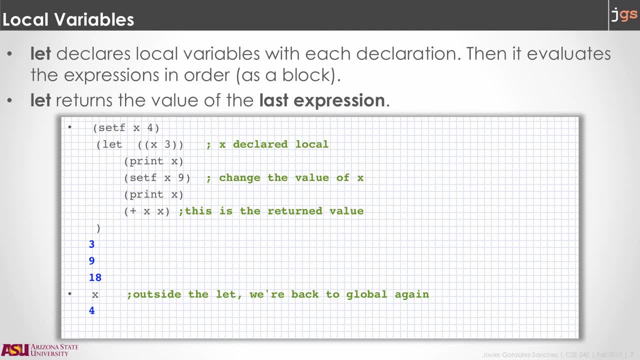 and now it's going to print 9. The return value in the let expression is going to be 18 and that is the last number printed on the screen. just because the last instruction is the addition of x plus x, 9 plus 9, In this example we define also a location x outside of the let. 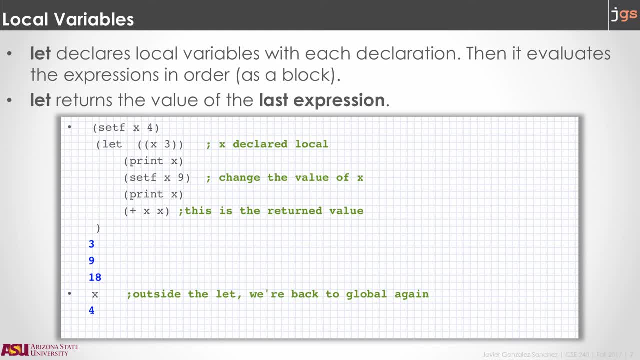 and we store the number 4 After the let expression. if we ask for the value in the location x, the interpreter is going to show us the number 4. that is the same value that we had before the let expression. so everything that we did with x. 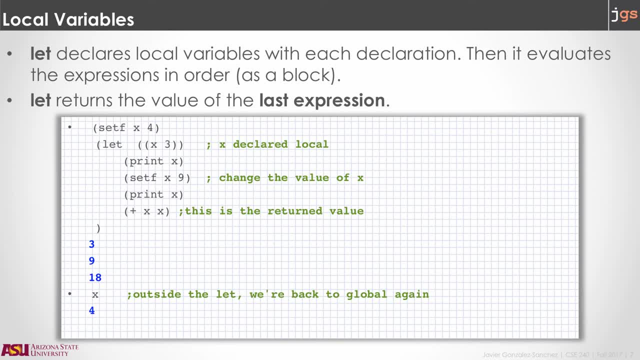 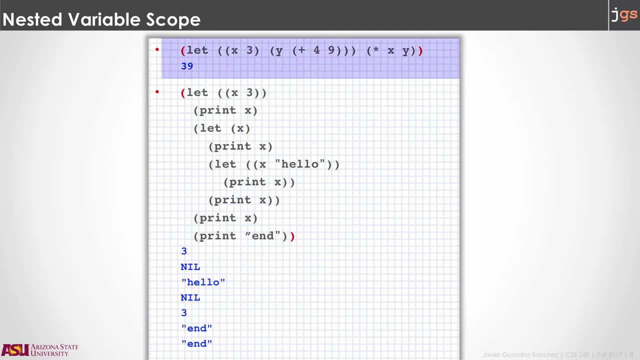 in the let expression is like working with a local variable. Here we have another two examples of let. the first one is: use one line. let is defining two symbols, x and y. for x the value is 3, but for y the value is the result of 4 plus 9. 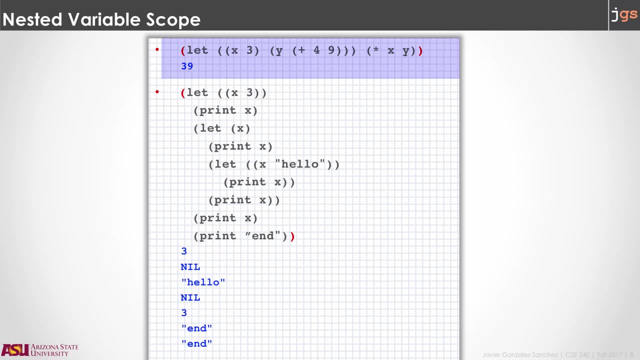 so you have the parentheses that enclose the function plus, that enclose the definition of y, the parentheses that enclose the definition of x and the parentheses that enclose both the definition of x and the definition of y. then you have only one instruction in this let expression. 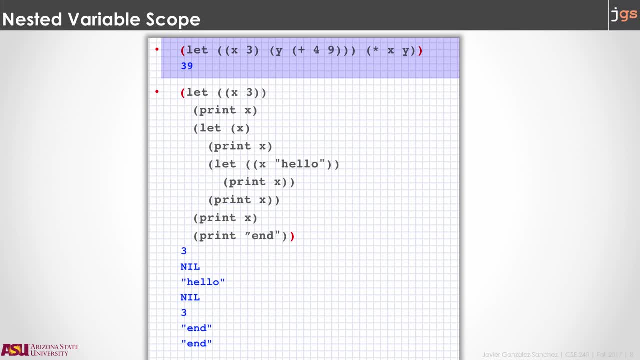 and that instruction is a multiplication, and it's a multiplication in which you use the variable x and y that you defined before. so the value for x was 3, the value for y was 4 plus 9, 13, so finally 3 times 13. 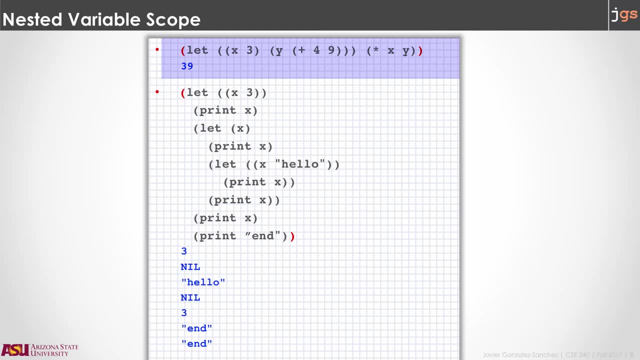 is equal to 39 and that is the result of the full expression. in the next example we are defining only one symbol, x, with the value 3, but notice that we have the parentheses for the list with the variables and also the parentheses for the definition of x. 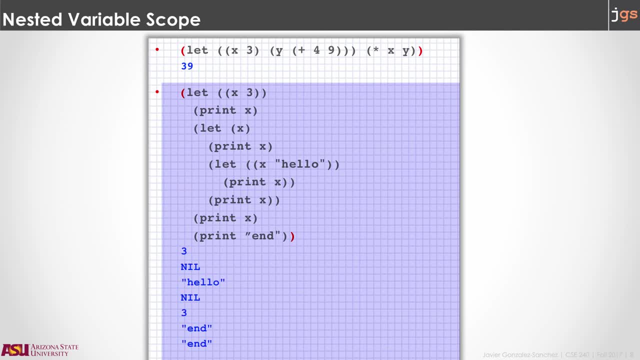 then we have one instruction- print x- and the second instruction is using again let. so we have something similar to a block inside of a block. in this new block, we define x. however, we didn't include a value for x. therefore, when you print x, it's going to print nil. 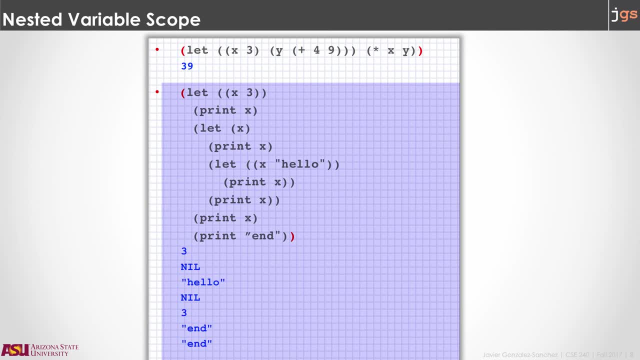 because we do not define a value for that instance of x. then again another block, another let, and here we define x with the value hello. so if you print that, it's going to print hello, and then we close that let expression. and if we try to print x again, 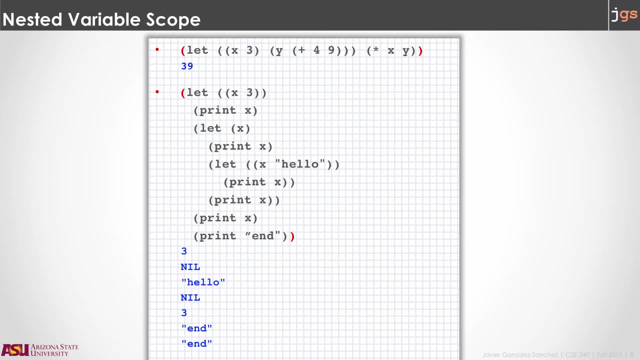 we are back to the value nil, closing that let. printing x again is printing again the tree that we have, that we have in the full expression of let and finally, the print n is printing n but also is the value that the full example is going to return. 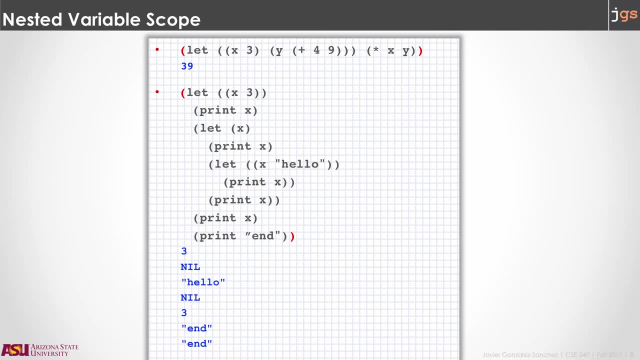 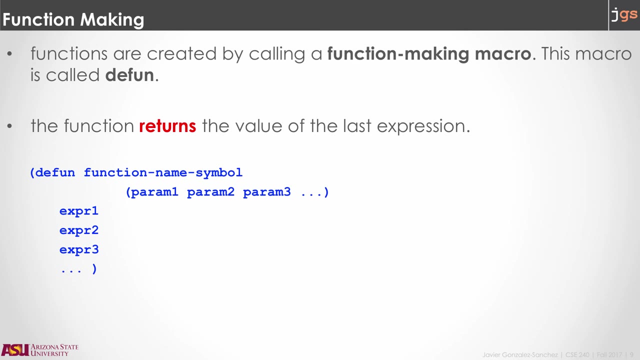 so you are going to saw n printed twice. in an imperative programming language, the example could be something like this here, if you know what it is, the entire number of value is going to be 1. 1, 1, 2, 3, 4, 5. 6, 7, 8, 9, 10, 11, 12, 13, 14, 15, 16, 17, 18, 19, 20, 21.